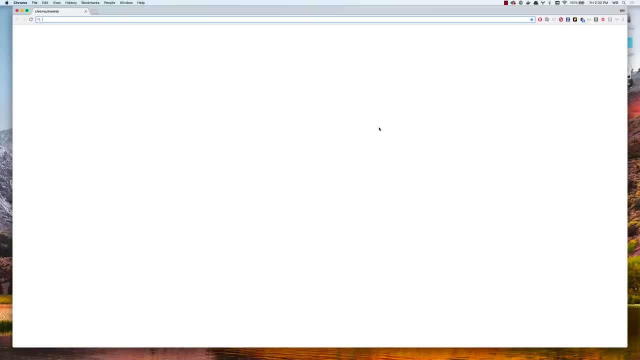 Hi there, my name is Will Stern and I've been a professional web developer for almost 20 years and in this course we are going to learn professional web development absolutely free, from the very beginning. My previous course on this on YouTube has had millions of views, thousands of comments, and I've 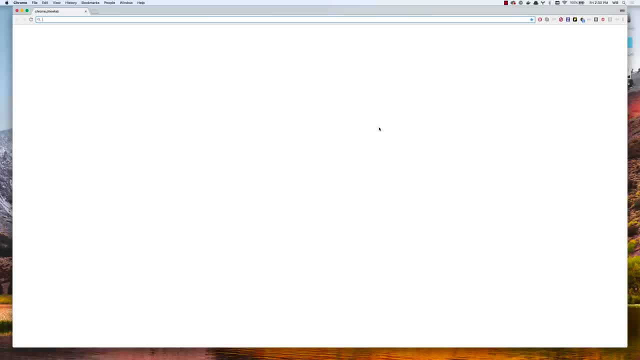 learned a lot about the common hang-ups people find and run into when they're learning web development. So we're gonna redo this course for 2018-2019, give you the most modern skill set to get you a career as a web developer. We're gonna 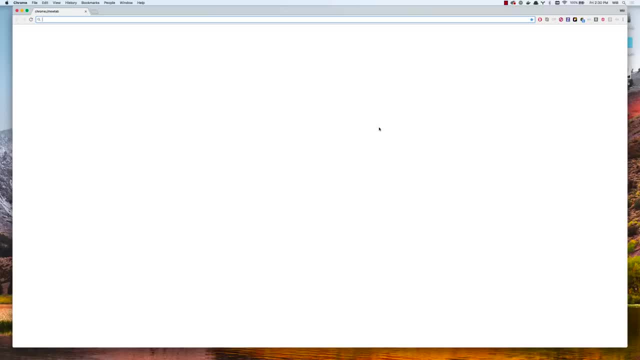 make it easy, fun and hopefully help you to avoid any confusing pitfalls that are common for people to end up with along the way. Now I want to mention really quickly, before we get into this course, that if you're here because you just need a website for yourself or for your business, you do not want to learn all of 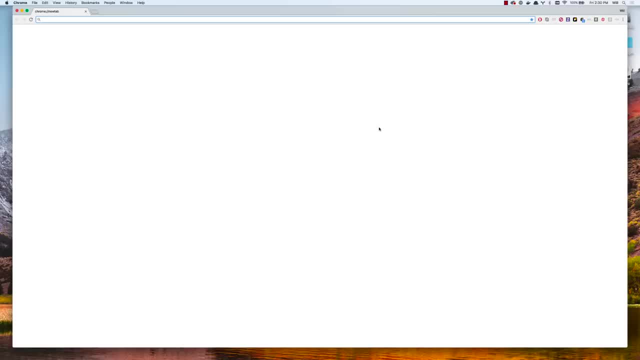 this. It's not the right road for you. Instead, look in the description. I have a link down there for the Wix ADI. That's their artificial intelligence web development tool and it's basically, with a few questions, going to build a whole. 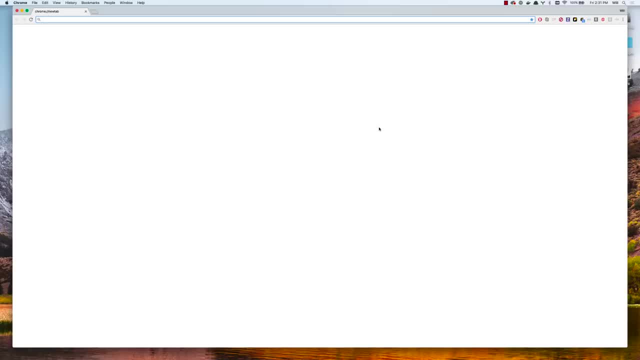 website for you that you can then custom. that is the fastest and cheapest way to get your website up if all you want is a website, If that's not you and you want to learn web development because you know how great of a career it is- and it is a great career with good pay and tons. 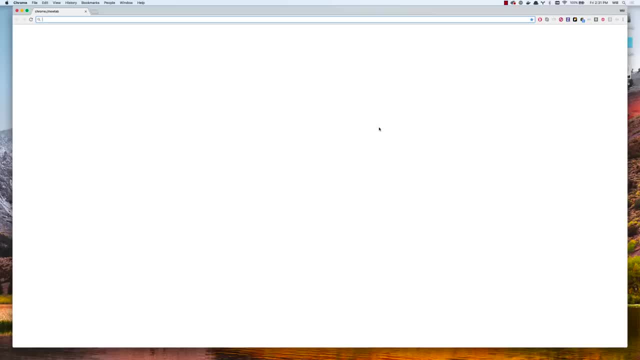 of demand, then let's get into developing websites and being a web developer in this day and age. So the first thing you'll need to do is let's install some professional web development tools. Good news, they're all free, because web developers love free stuff. So what I want you to do is open your web browser. 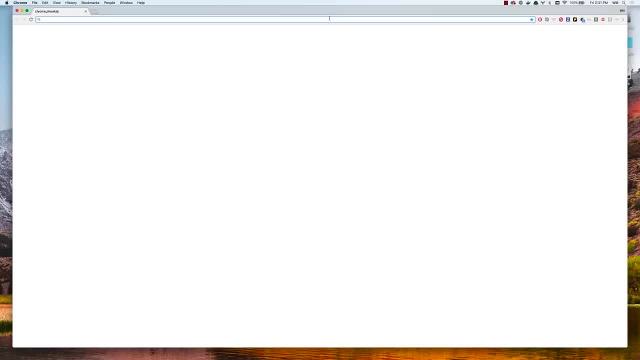 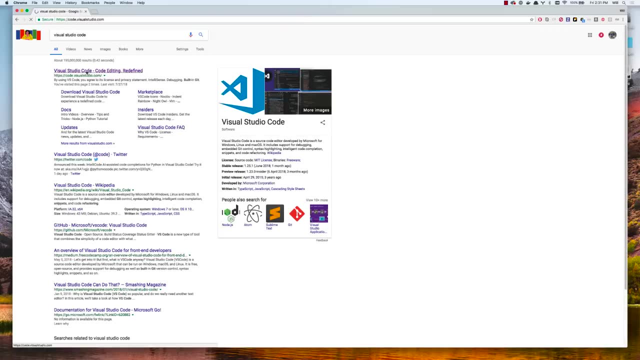 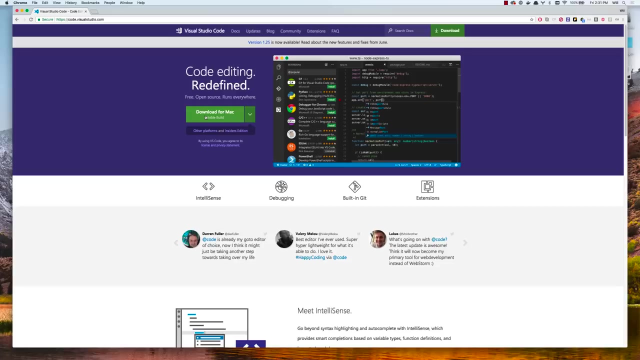 which I prefer- Chrome and most web developers do these days. But open your web browser and go to Visual Studio Code. just Google search Visual Studio Code and that's gonna take you to this, and I want you to download it. This is the best web development tool out there that is free. Not everybody uses the same text. 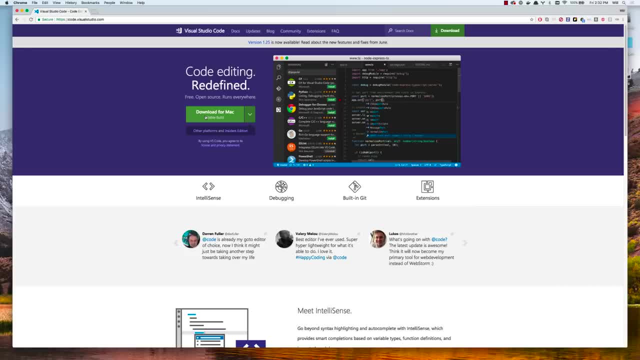 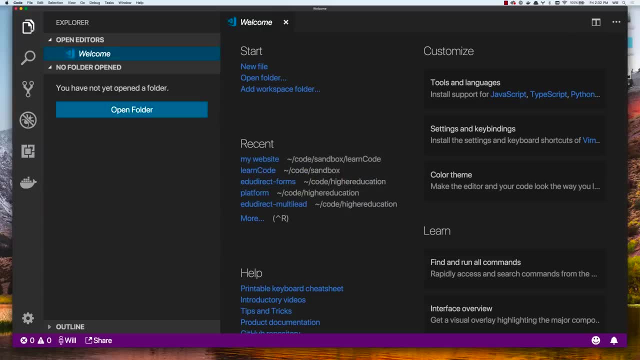 editor, but Visual Studio Code is probably the most popular text editor these days, So go ahead, download it, install it, start it up and you'll end up with something like this studio code right here, although you'll probably see a welcome screen that looks: 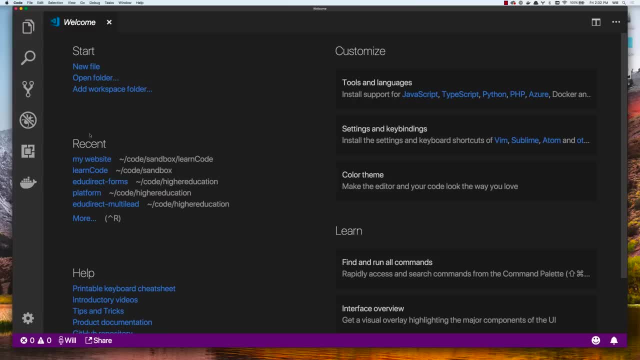 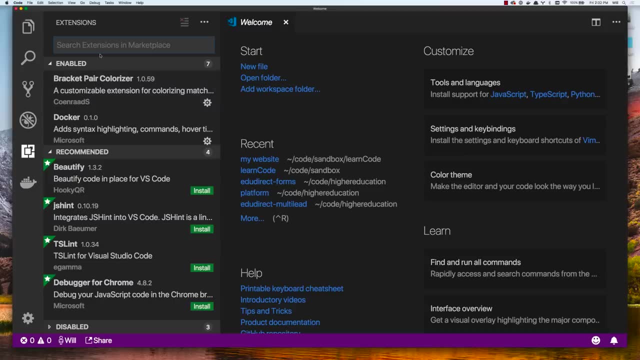 like this. now I want you to install one thing. once you get it open, I want you to click over here onto this square button and you can install all these great extensions for free from the marketplace, and the one that we're the most interested in right now is called live server. so go ahead, search for live. 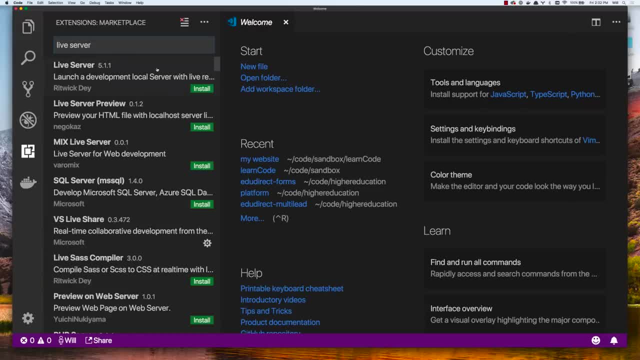 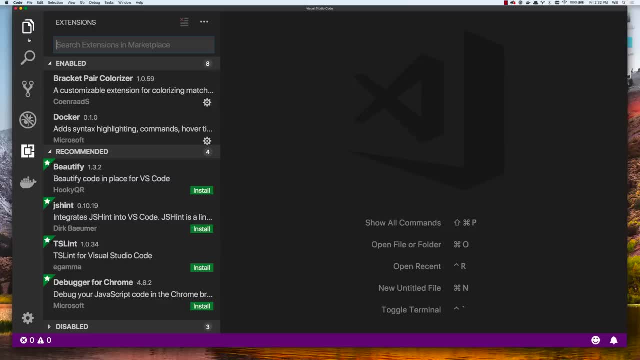 server and get this top one right here. launch a development local server with blah blah- yes, install that. we want to install that- and reload, and you'll see in just a second what that does for us. so now that live server is installed and we have Visual Studio Code installed, we're ready to start coding. this is 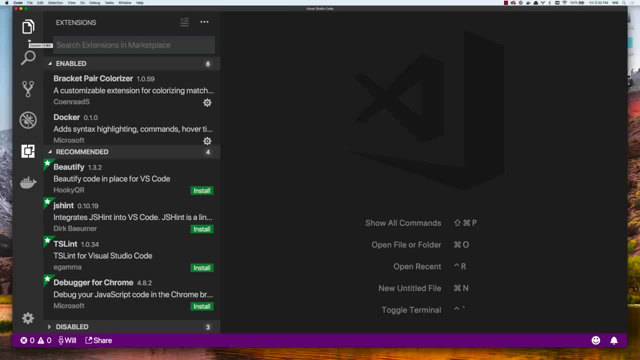 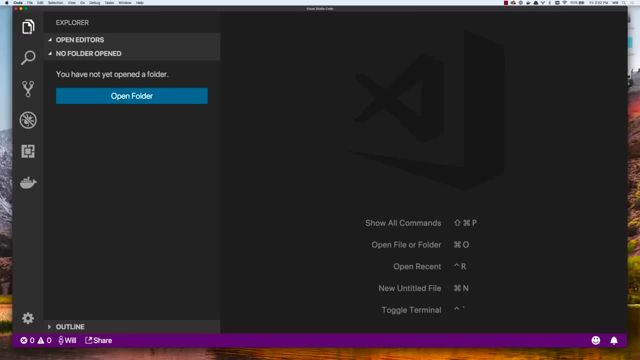 exactly what professionals see all day, every day, when they're coding is Visual Studio Code or the text editor of their choice if they don't want to use Visual Studio Code, so let's make a project and create our first super ugly, super basic website. before we wrap up this tutorial, I want you to go over to this files tab. 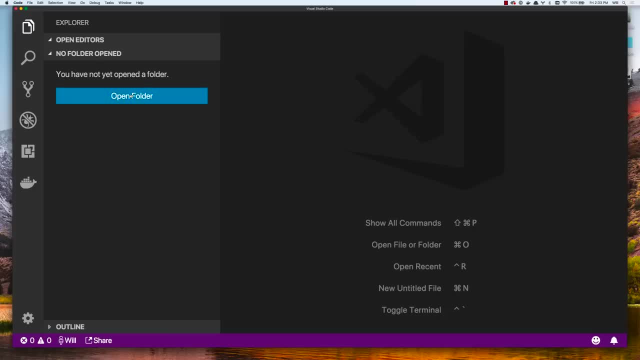 here and click on it and you can see it says: hey, you haven't opened a folder yet. you can see it says: hey, you haven't opened a folder yet. you can see it says: hey, you haven't opened a folder yet, let's go ahead and open a. 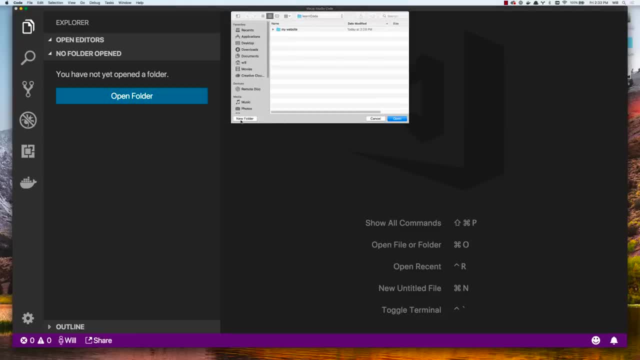 let's go ahead and open a folder. in this case, you get to choose where you want to. let's go ahead and open a folder. in this case, you get to choose where you want to go. maybe create a new folder somewhere? in this case, I already have a folder. 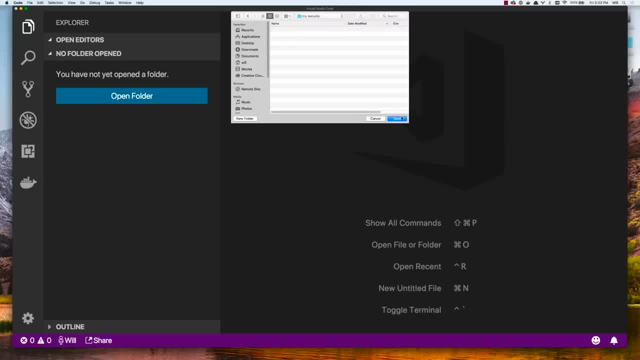 go, maybe create a new folder somewhere. in this case, I already have a folder called learn code and I have a folder called my website, so I'm going to use called learn code and I have a folder called my website, so I'm going to use this one- and then in this folder you want to create your very first file. 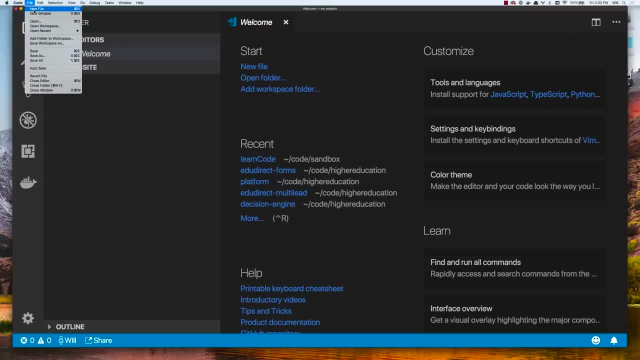 this one and then, in this folder, you want to create your very first file, which you can do the new file button. or you can go file new, or you can just do. which you can do, the new file button. or you can go file new, or you can just do. 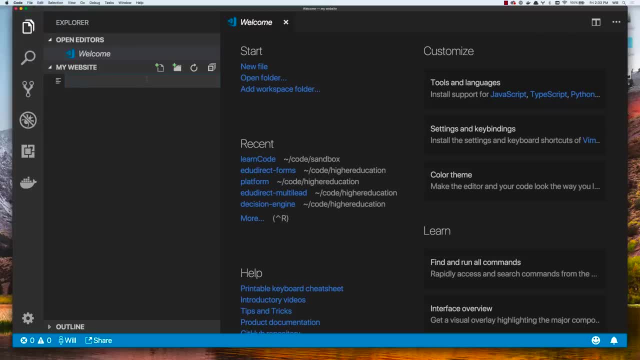 command N or control, and if you're on a command N or control, and if you're on a command N or control, and if you're on a PC, so let's go create our new file. we PC, so let's go create our new file. we PC, so let's go create our new file. we always want to call this first file the. 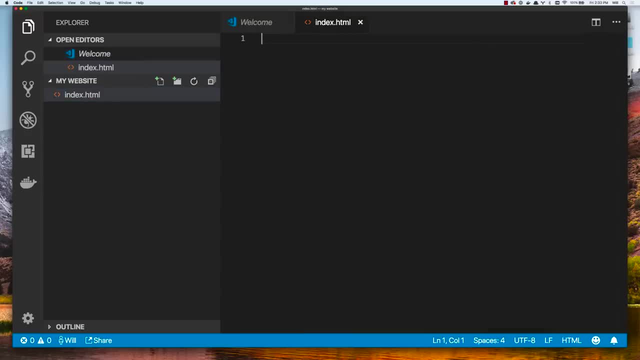 always want to call this first file. the always want to call this first file the homepage of our website index. HTML homepage of our website index. HTML homepage of our website index. HTML index is what the website is index. is what the website is index. is what the website is automatically going to open when you go. 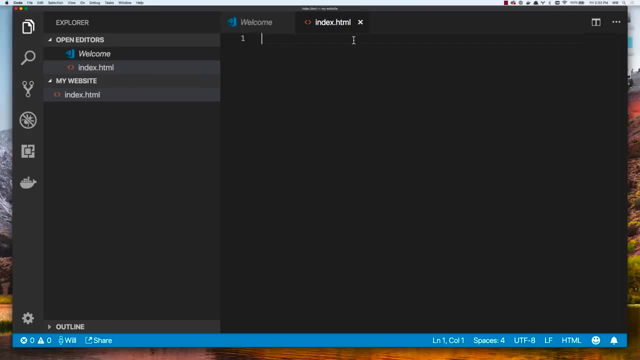 automatically going to open when you go. automatically going to open when you go to your awesome website com. so here we to your awesome website com. so here we to your awesome website com. so here we have index dot HTML and I want you to do. have index dot HTML, and I want you to do. 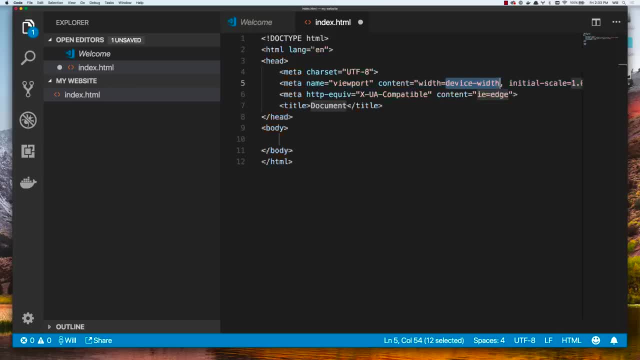 have index dot HTML and I want you to do something really sneaky here. just hit something really sneaky here. just hit something really sneaky here. just hit exclamation mark and then hit tab and exclamation mark, and then hit tab and exclamation mark and then hit tab and boom. don't freak out, this looks like a 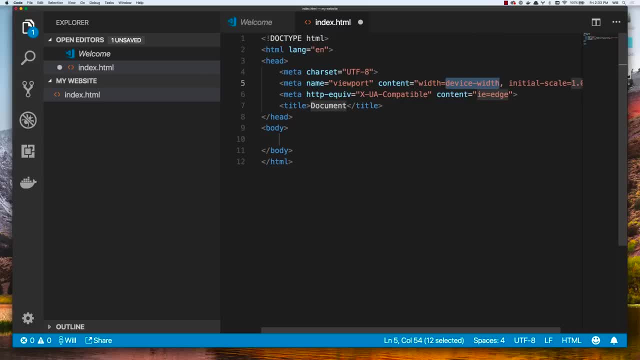 boom. don't freak out. this looks like a boom. don't freak out, this looks like a lot of code, but it's actually not lot of code. but it's actually not lot of code, but it's actually not confusing at all. we with exclamation tab. confusing at all. we with exclamation tab. 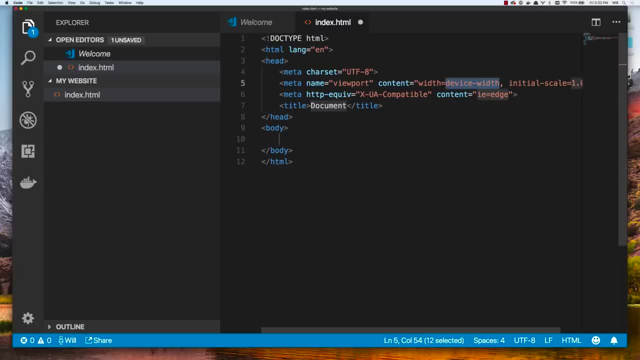 confusing at all. we, with exclamation tab, we created the empty website template. we created the empty website template. we created the empty website template. what you want to do is go in between. what you want to do is go in between. what you want to do is go in between these two body tags: body tag and body. 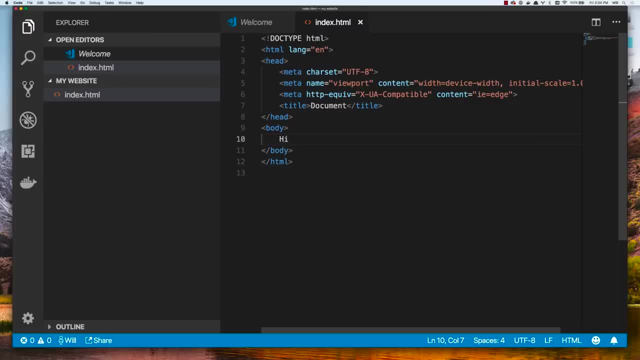 these two body tags- body tag and body. these two body tags- body tag and body tag. and go ahead, say something. let's say tag, and go ahead, say something, let's say tag. and go ahead, say something. let's say hi and hit save. you'll want to learn to. 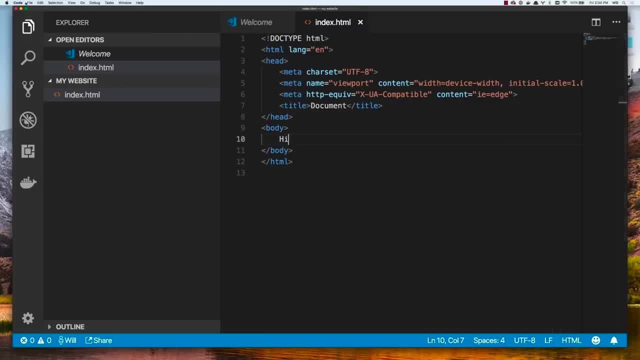 hi and hit save. you'll want to learn to hi and hit save. you'll want to learn to hit save from your keyboard. which on a hit save from your keyboard. which on a hit save from your keyboard. which, on a Mac, is command s or ctrl s from Windows. 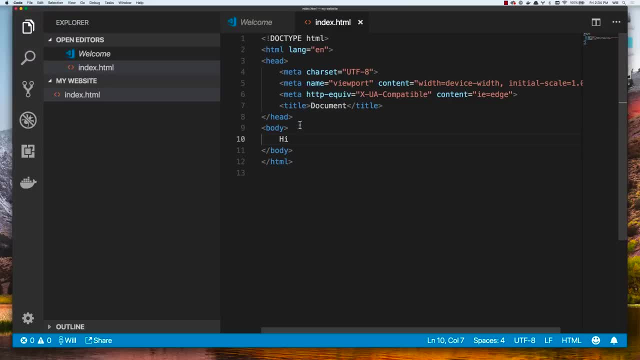 Mac is command s or ctrl s from Windows. Mac is command s or ctrl s from Windows. or you can just do file save, but that's, or you can just do file save, but that's, or you can just do file save, but that's a lot slower. you're gonna want to save a? 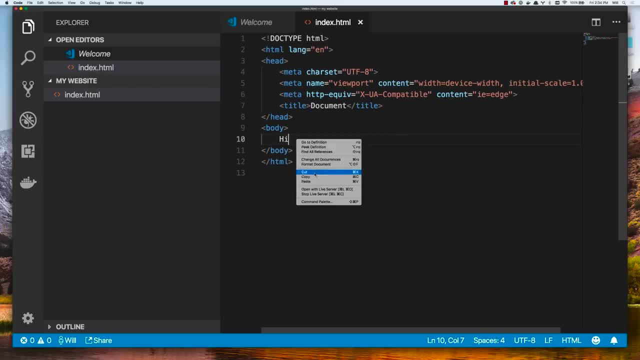 a lot slower. you're gonna want to save a a lot slower. you're gonna want to save a lot once you've saved your page lot. once you've saved your page lot. once you've saved your page, right-click and click open with live. right-click and click open with live. 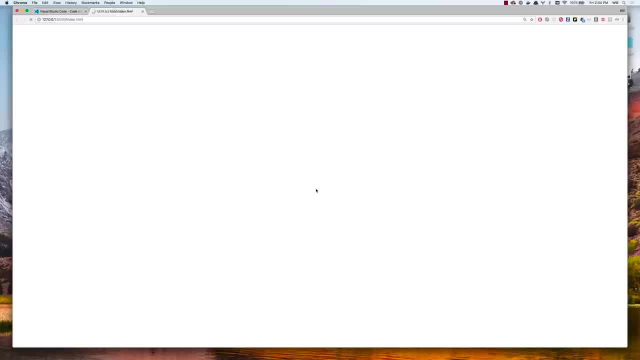 right-click and click open with live server. you should have this because you server. you should have this because you server. you should have this because you created your live server, or you install created your live server, or you install created your live server, or you install live server. so now you can see, I've got. 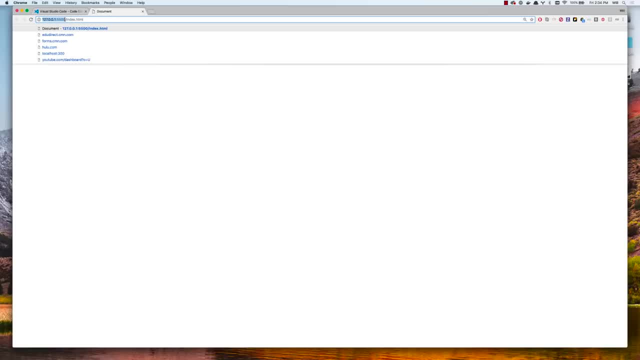 live server. so now you can see I've got live server. so now you can see I've got this live server that it created on my this live server, that it created on my this live server, that it created on my machine instead of a website, and it's. 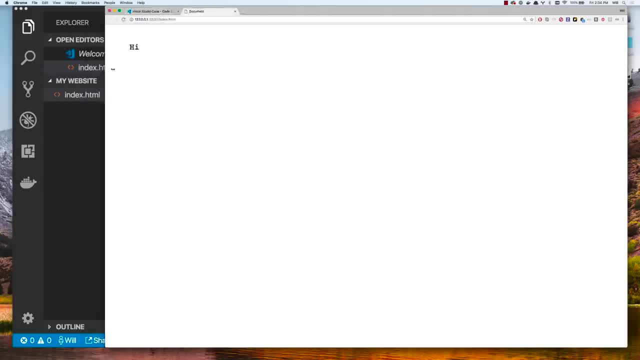 machine instead of a website, and it's machine instead of a website and it's going to index dot HTML. and there's my going to index dot HTML, and there's my going to index dot HTML. and there's my website. hi, what I can do now is I can. 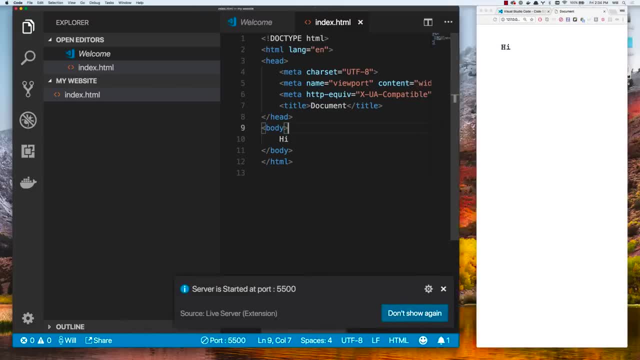 website hi. what I can do now is I can website hi. what I can do now is I can kind of create a layout here by dragging, kind of create a layout here by dragging, kind of create a layout here by dragging my two windows so I can see them both at. 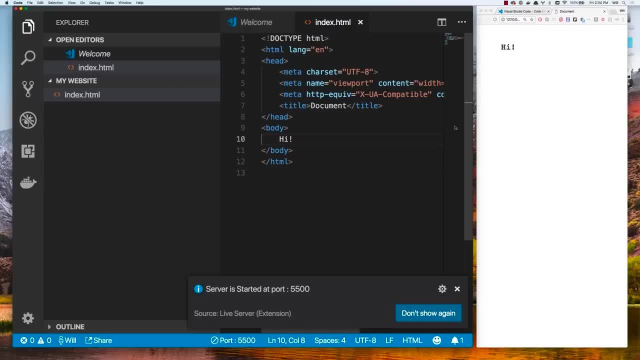 my two windows so I can see them both at my two windows, so I can see them both at once. and if I change this, maybe add an once. and if I change this, maybe add an once. and if I change this, maybe add an exclamation mark. and it's safe it. 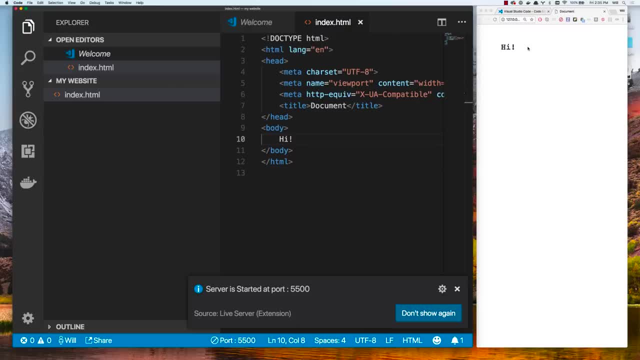 exclamation mark and it's safe. it exclamation mark and it's safe. it automatically reloads. that's because my automatically reloads, that's because my automatically reloads, that's because my live server is doing something called live server is doing something called live server is doing something called live reloading, where, whenever my, my, 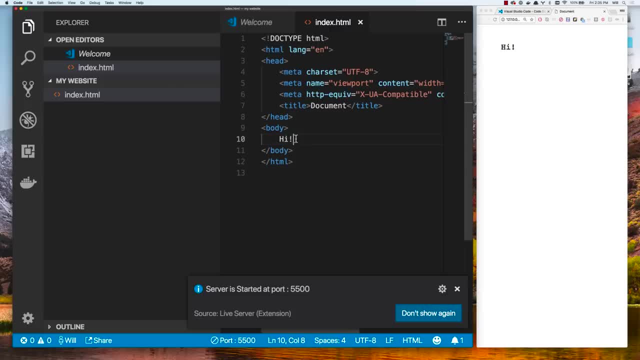 live reloading, where, whenever my my live reloading, where, whenever my my website changes, I get to see that change website changes. I get to see that change website changes. I get to see that change right away. it's a great development right away. it's a great development right away. it's a great development experience. so I can say: hello, world hit.